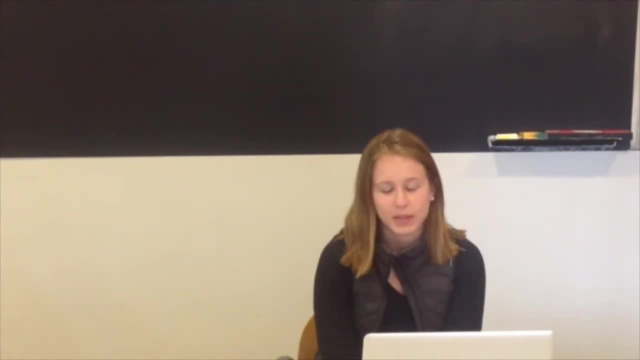 kinds of investments and why it ought to promote environmental protection in its work. To understand sustainable development, we must first understand that the well-being of the economic system is intrinsically tied to the well-being of the environment. The economy's functioning depends on inputs from nature, which are then exchanged among various market actors, and 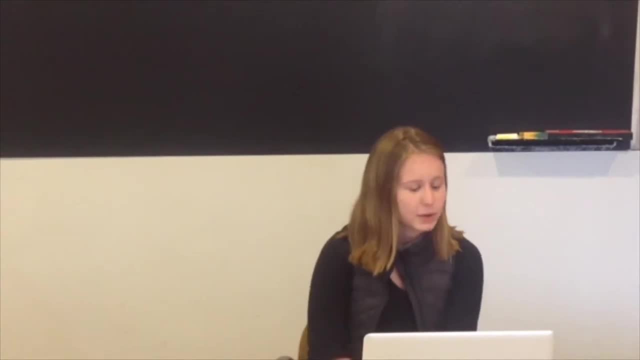 eventually output as waste into the environment. The economy grows at an unsustainable rate when the rate of resource consumption and waste production exceeds the rate at which the environment can regenerate and absorb waste products. It is also important to note here that economic growth is simply a measure of total resource throughput. It says nothing. 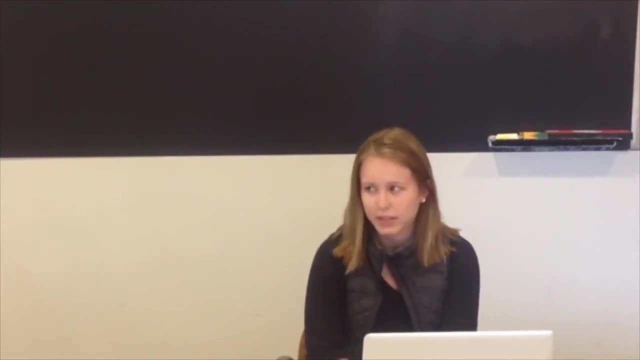 about the happiness, health, safety or sense of community within a region. Now that we have defined growth, we can contrast it with the concept of development. Development is the qualitative improvement of resource efficiency within a region. To invest in projects that promote development in poor countries is to invest in projects that allow people to produce. more with the resources they need. To invest in projects that promote development in poor countries is to invest in projects that allow people to produce more with the resources they already have. These kinds of projects may involve investing in education, investing in the construction of local hospitals and clinics, or investing in research and development. 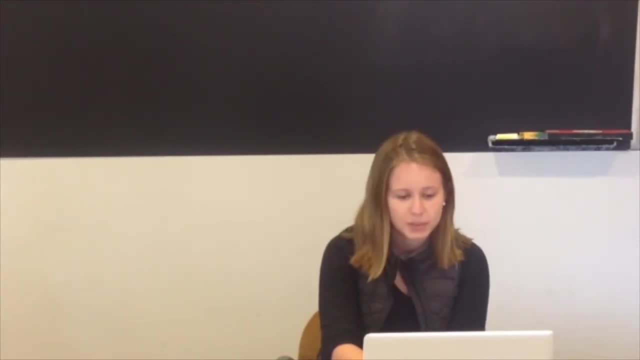 of crop seeds that are less resource intensive. While projects that promote growth simply increase production and consumption, projects that promote development increase efficiency in production and consumption towards some end that enhances human welfare. Economic growth is less important than economic development because growth, in other words, is a process. 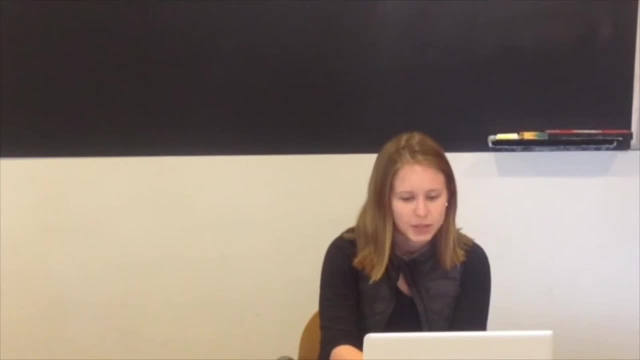 of business development, usually measured in terms of GDP, is a flawed measure of progress. There is nothing inherently beneficial about economic growth. This is because growth only implies an increase in resource throughput. It doesn't take into account whether the resources are being used in ways that efficiently maximize well-being while minimizing resource consumption. 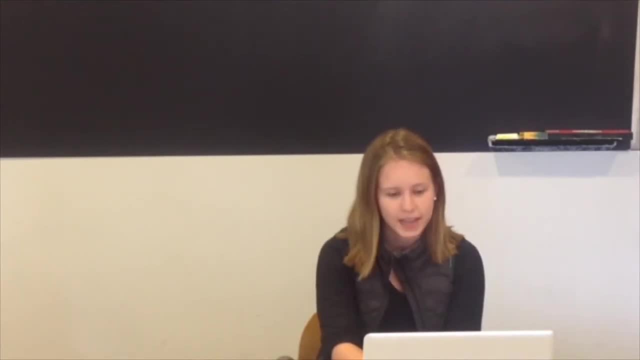 On the other hand, economic development does a far better job of indicating economic progress. Development implies that resources are being used in increasingly efficient ways. The more developed a country is, the more it benefits from the resources it has, while minimizing its total consumption of these resources. 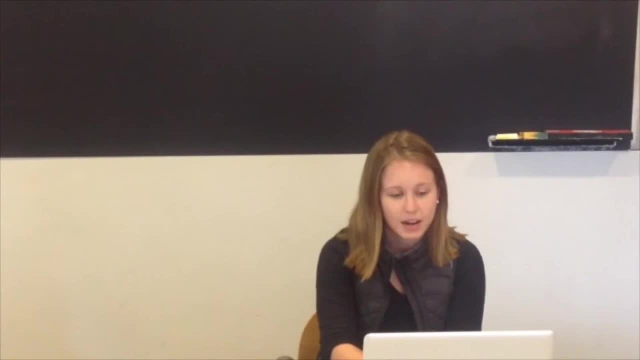 As it becomes more and more clear to people across the world that development, not growth, should be our top priority, then the bank's investment goals will be in line with the goals of the rest of the world. This is because investors will want the same thing as anyone else: the maximum amount of benefit they can get at the lowest cost. Likewise, individuals who recognize development as their goal want to receive the greatest benefit from natural resources which they use, while minimizing resource consumption. As the UN's international financial institution, the World Bank's mission is to reduce poverty. It should do this by promoting economic development which ensures the long-run integrity of economic systems. 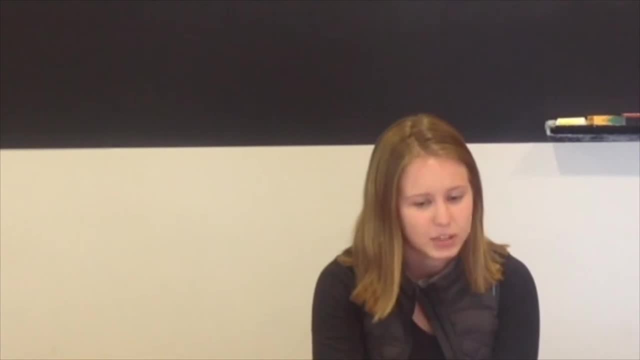 If the bank instead chooses to promote economic growth, it will be investing in projects that contribute to constructing an unsustainable economic and social paradigm with incredible inertia. The longer economic growth remains the dominant measure of progress, the more difficult it becomes to achieve its goal. 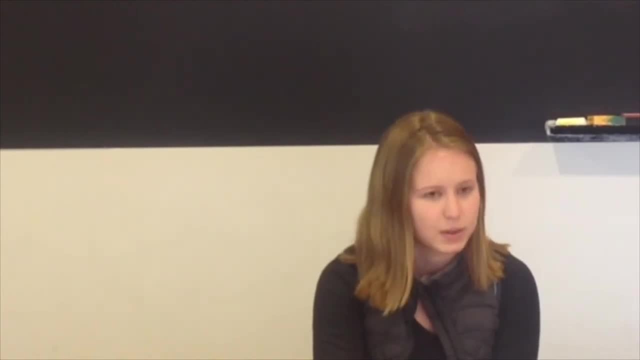 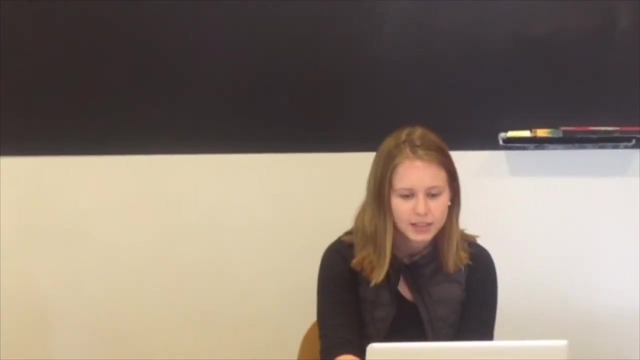 It will be to change our consumption patterns in business practices to ones that are more sustainable. The World Bank need not look very far in seeking out philosophical justification for taking this measure. Utilitarianism, the common philosophical foundation for much of existing environmental policy, tells us that we should take the forward-looking, utility-maximizing action. 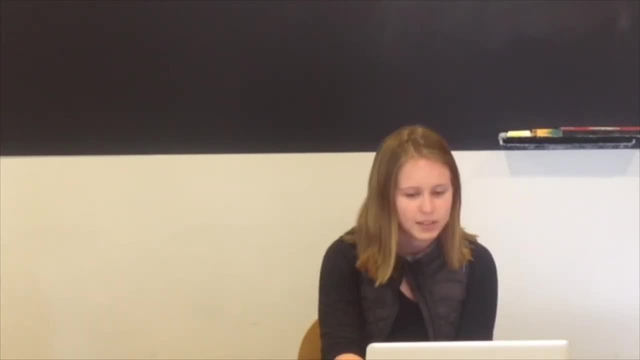 Choosing to make investments that promote development, not growth, is just such an action. This is because human well-being in the long run is maximized from the very beginning. The very goal of the economic system is to provide for human needs while maintaining the integrity of the environment in the long run. 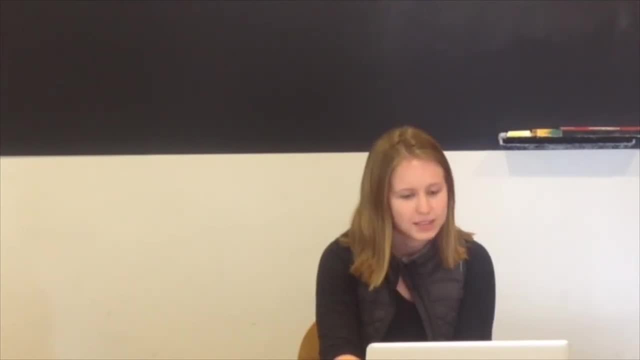 Human welfare is certainly not maximized when the goal of the economic system is to simply maximize consumption, without regard to the system's long-run viability. Such economic growth reduces our collective welfare because it leads to depletion of economic inputs, natural resources that are used as raw materials, as well as the accumulation of economic outputs, which are manifested by landfills and garbage packs. 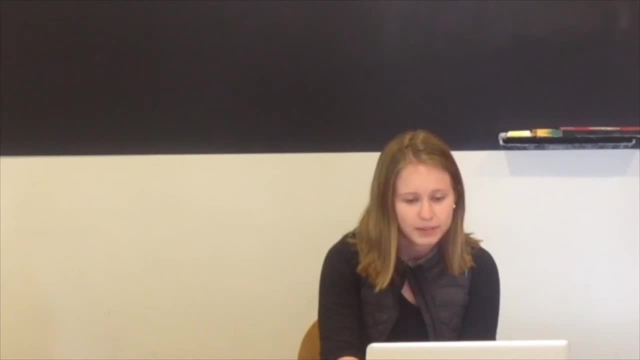 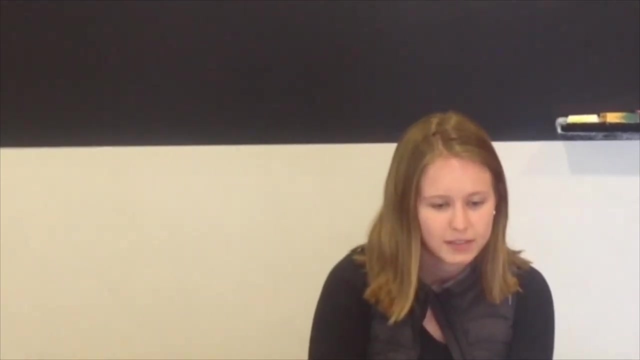 Neither of these outcomes are ones that anyone would want. If the World Bank's goal is to reduce poverty in the long run, it must take a long-run view of success. As a UN initiative with a moral imperative, the World Bank should work to ensure that its investment decisions are based on a utility-maximizing philosophy that promotes long-run human welfare. 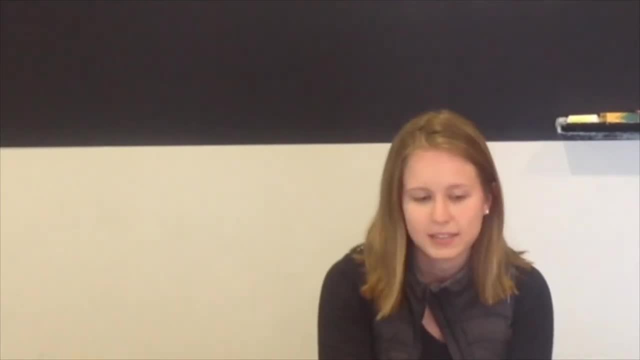 Indeed, investments in development-related projects pay dividends over many years, while investments in growth-related projects may only provide for human needs for the long run. It is the World Bank's responsibility to take into account the long-run well-being of the environment, because the viability of economic systems depends on its sustained integrity. 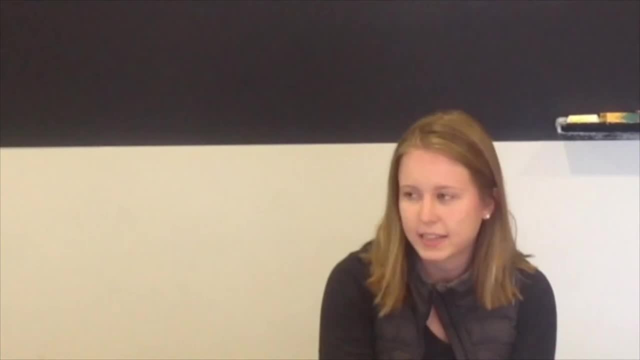 To promote growth is to promote the idea that the economy can continue to flourish independently of the environment, an idea that is a fiction. However, to promote development means to promote human progress that is sensitive to the environment's carrying capacity and actively works to promote environmental stewardship.